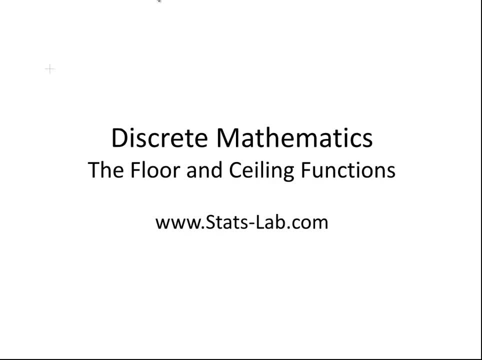 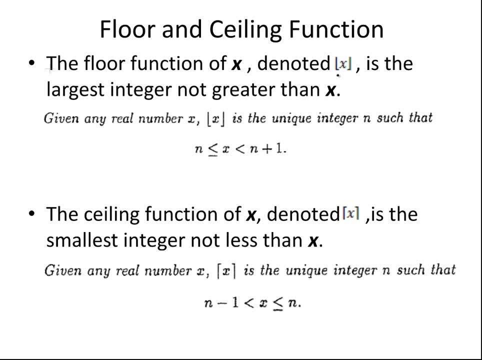 In this presentation we are going to look at the floor and ceiling function, So the floor function of x, which we will denote with this symbol. here it is a square bracket missing. the top component is the largest integer not greater than x. So the largest integer not greater than x. 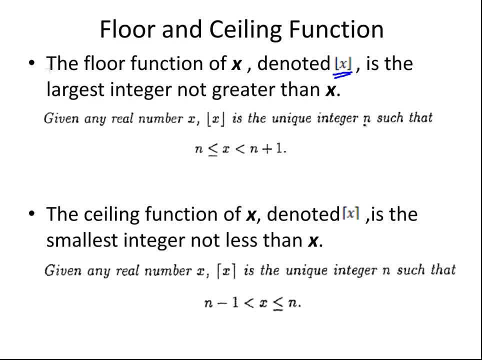 Given any real number. the floor function is unique integer n, such that n is less than or equal to x. We are not really that particularly concerned about the rest of that expression. The ceiling function of x, which we will denote there again- this time in the square brackets the bottom part is missing- is the smallest integer, not less than x. 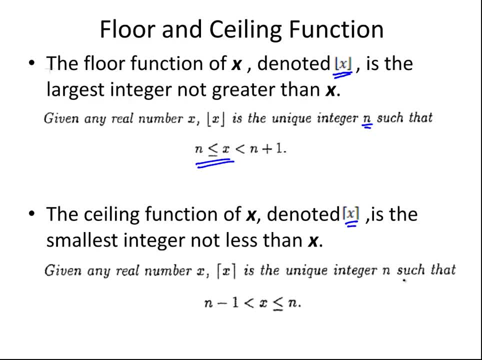 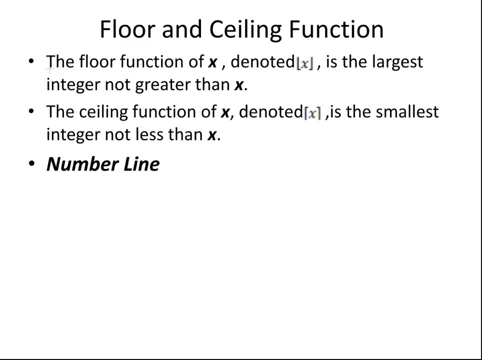 So, given any real number, x, the ceiling function is a unique integer, n, such that x is less than or equal to n. So n is an integer. So floor and ceiling functions, the outcomes, are integers. So the floor function of x is ok. sorry, this is what I want to look at here. 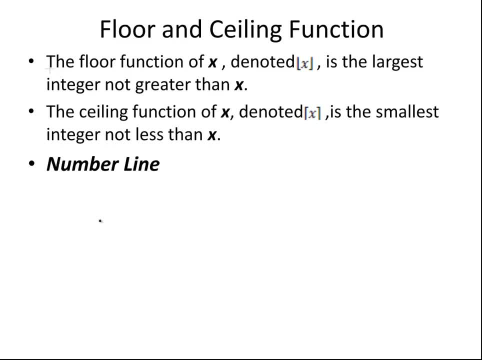 This is a number line, So I am just going to draw a straight line here. And that is not a straight line, Give me another, go there. So there we go. Now I am going to pick. this is going to be the zero point. 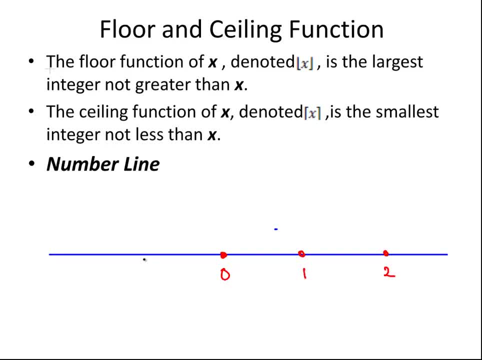 Make this 1.. 2. And I am going to go minus 1 and minus 2 here. So this is the number line. Those are all integers. What I am going to do is pick out two points. I am going to pick, let's say, 1.3.. 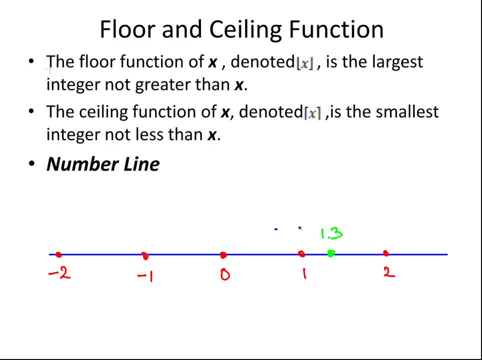 Well, the floor function of 1.3 is 1.. It's the integer that precedes it on the number line And the ceiling function of 1.3 is 2.. It's the integer that comes next in the number line. 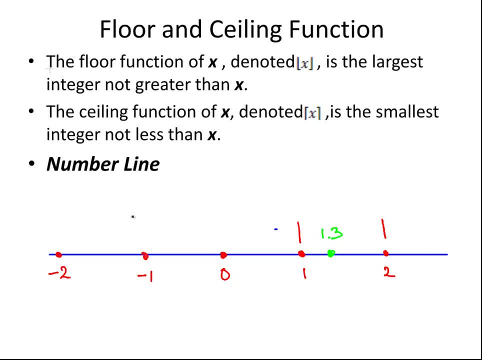 So ok, Now let's go to the other end here. Let's suppose we are dealing with minus 1.5. let's say Now, this is be very careful here, And it's actually a good idea to visualize the number line when you are doing these. 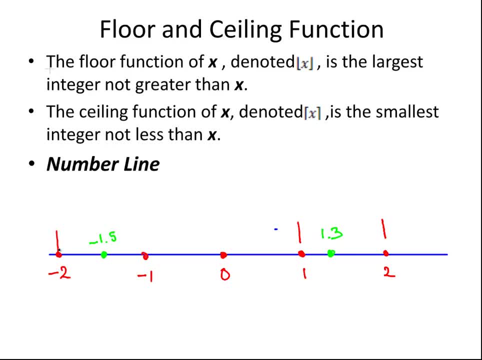 The integer that precedes it in the number line is minus 2.. And the integer that comes after it is Minus 1.. So that could be a bit very counter intuitive. So let's write that out. The floor function of 1.5 is minus 2.. 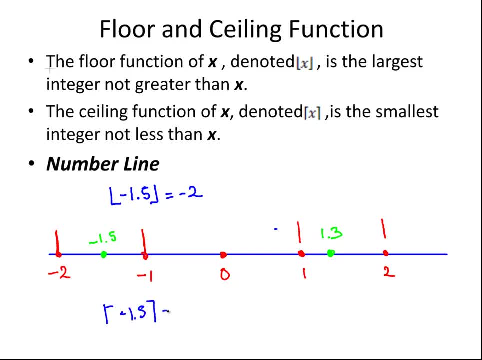 The ceiling function of minus 1.5 is minus 1.. Likewise over here, the floor function of 1.3 is simply 1.. The ceiling function of 1.3 is 2.. It's actually usually on the negative side of the number line that we run into. 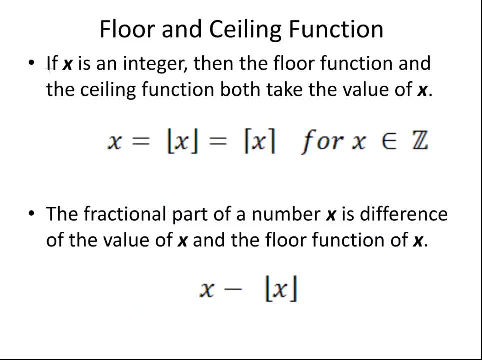 Problems. Ok, Now, if x is an integer, then the floor function and the ceiling function both take the value of x. So if x is an integer, x equals the floor function of x equals the ceiling function of x. Now, a useful sort of another extra sort of component that is brought into consideration when we are doing these type of problems. 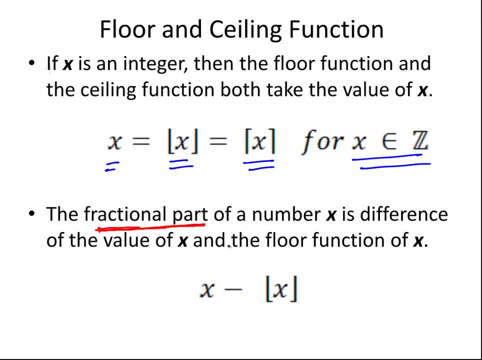 Is the fractional part of a number, x. It's the difference of the value of x and the floor. So we write it like this: x minus the floor function of x. Ok, Let's look at some examples here, So 2.4.. 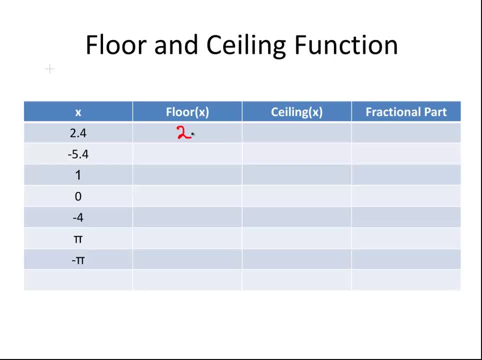 Floor function of that Is 2.. The ceiling, 3. And the fractional part 2.4 minus 2.. That is 0.4.. The floor function of minus 5.4.. Just remember the number line. 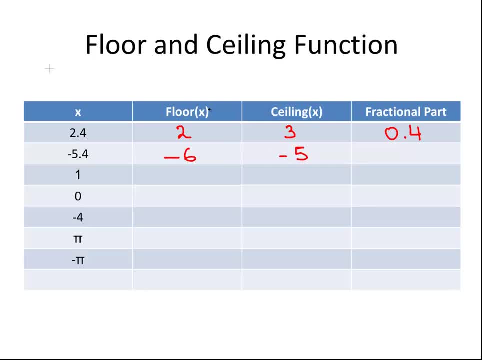 It's minus 6.. And in this case the ceiling is minus 5.. Now Let's do the fractional component here again. You might be surprised by this result: Minus 5.4, minus minus 6.. The minuses cancel out. 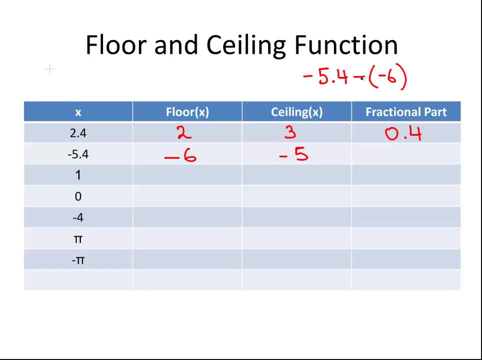 So actually, what we are left with is Plus 6, essentially. Let's just rub that out there So it actually becomes Plus 6.. Plus 6.. And the answer is therefore 0.6.. So the fractional parts can be again.